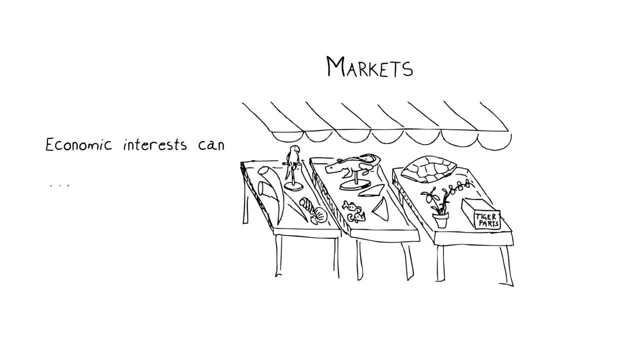 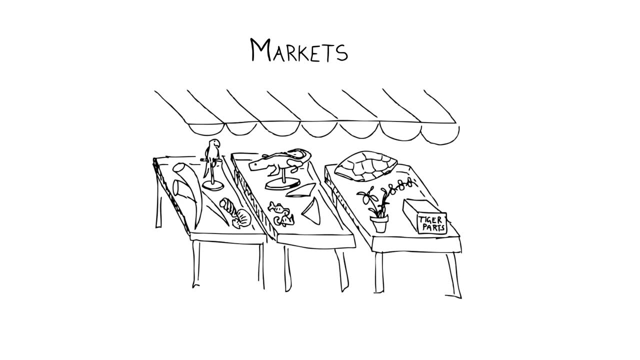 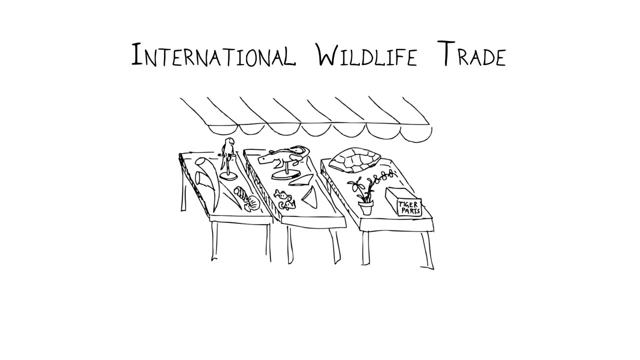 but to the markets themselves. an example of how economic interests can and should dovetail with protection of the environment. In some cases, a species is so threatened that a complete ban on its trade is required. International wildlife trade is estimated to involve hundreds of millions of individual plants and animals, resulting in a market worth billions of dollars. 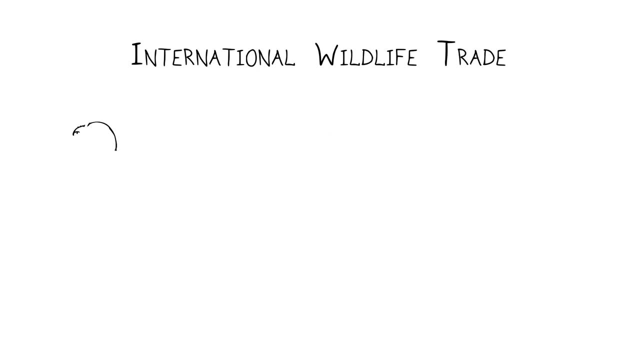 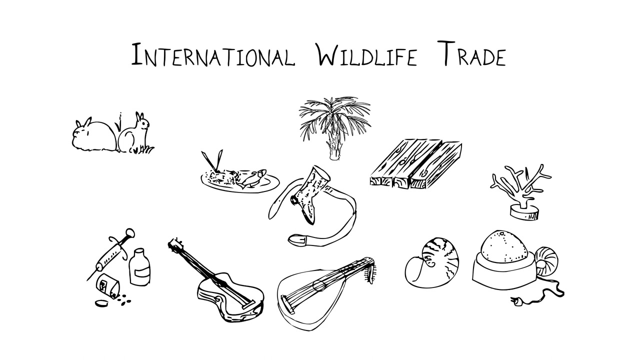 a year, So it's not a small problem, And it ranges from live animals and plants to products that are derived from organisms such as food, leather goods, timber, curios, medicines and even things like wooden musical instruments. Another really useful conservation tool is the Red List of the International Union for 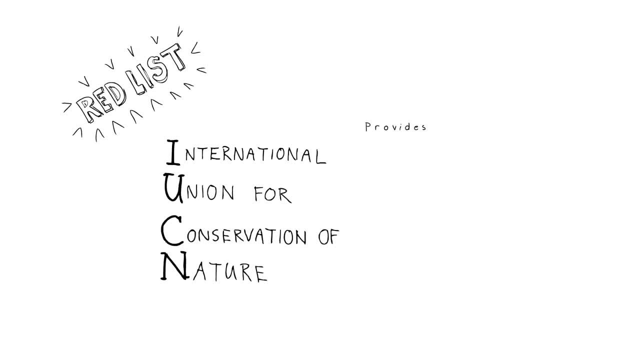 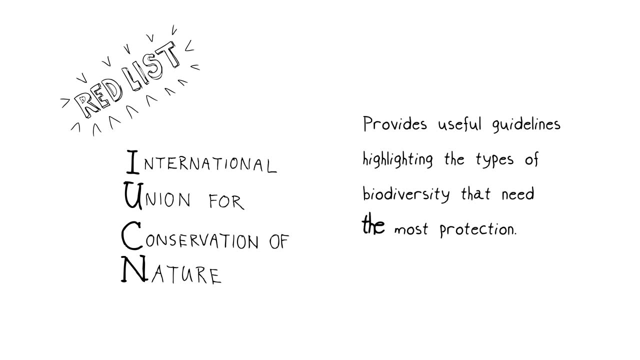 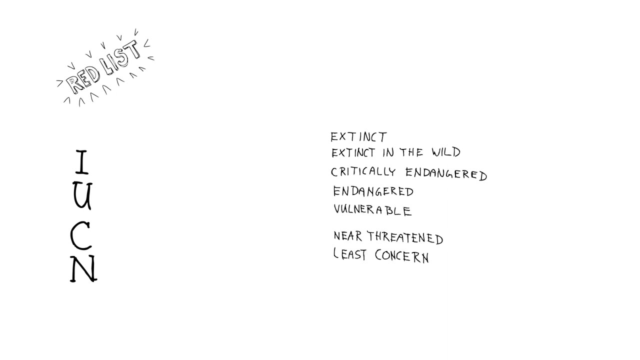 Conservation of Nature. This tool is used by researchers to study the population of the nature, the IUCN, which provides very useful guidelines highlighting the types of biodiversity or the species themselves that need to be protected the most. All species are placed in one of seven IUCN categories, ranging from extinct to least. concern Placing a species. 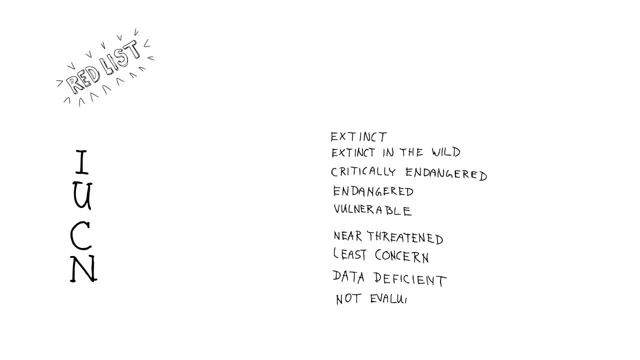 into these categories requires adequate data which underscores the importance of biodiversity research and the dissemination of life, And that's what I always mean about biodiversity research and its symbiotic partner education. Good data equal better decisions. The IUCN highlights the crucial nature of research. 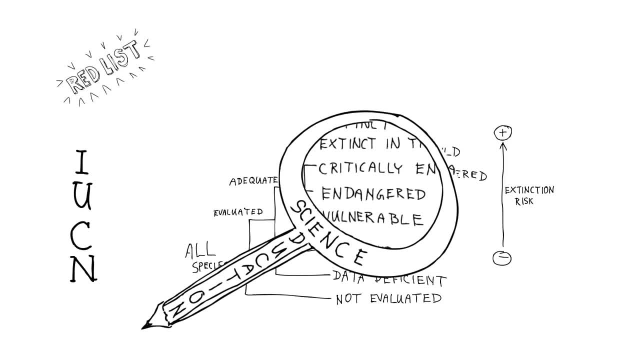 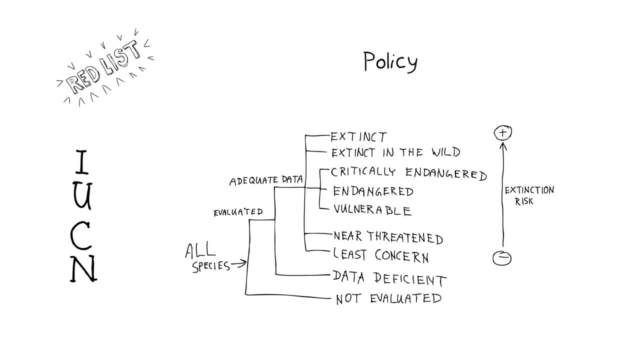 If you have the right data, you can place known species into one of the seven different categories, Categories that are really really helpful for education, as well as for making good protection policies and even for helping fundraise for more research, more education. 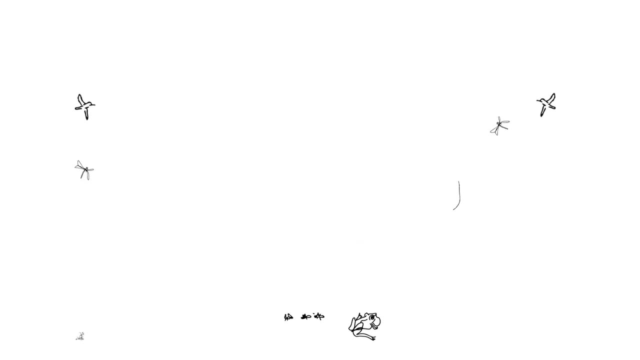 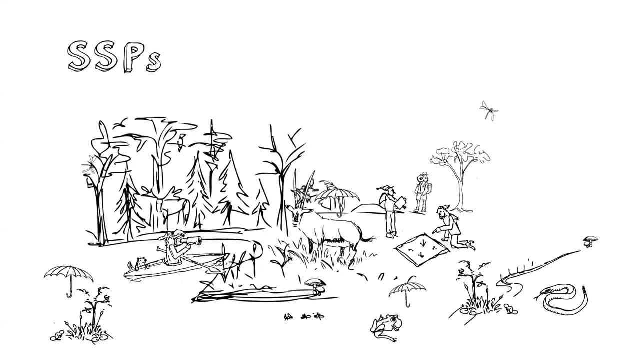 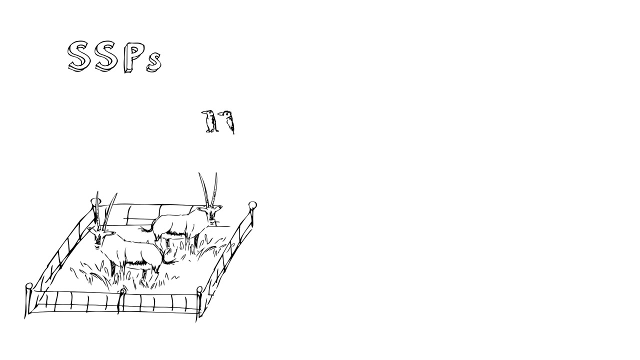 and conservation. Another species protection technique involves the establishment of Species Survival Plans or SSPs. When scientists believe that captive breeding programs can help prevent extinction, SSPs can be developed for species that are in danger of extinction in the wild. SSPs help to maintain in captivity a reservoir of healthy populations of endangered animal. 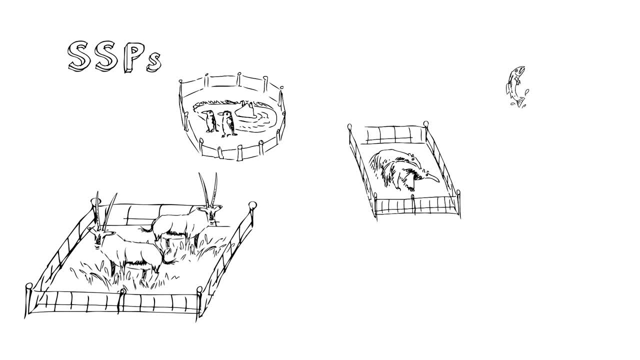 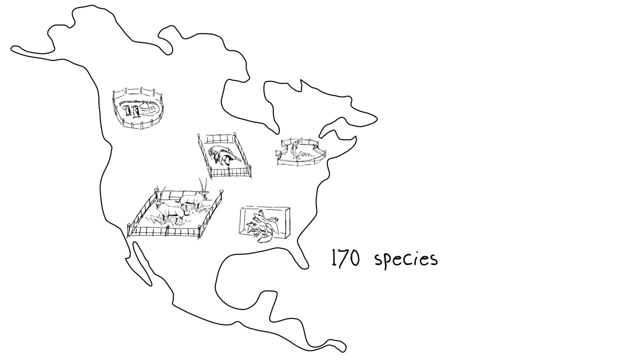 species Populations that maintain genetic diversity through careful breeding programs within the accredited community of zoos and aquaria that are approved for maintaining these breeding programs. In North America alone, there are over one hundred and seventy species covered by more than one hundred formal species survival plans that are specifically 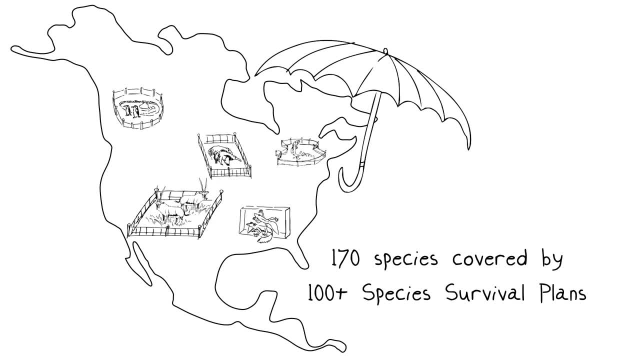 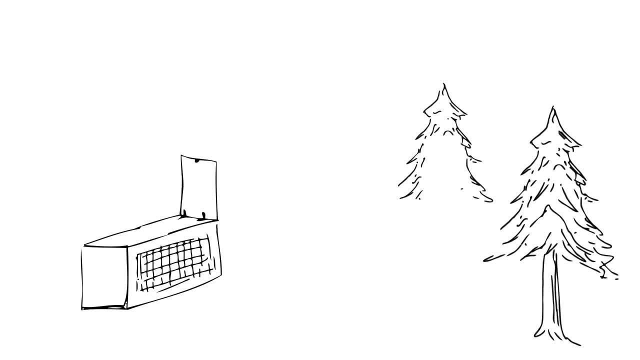 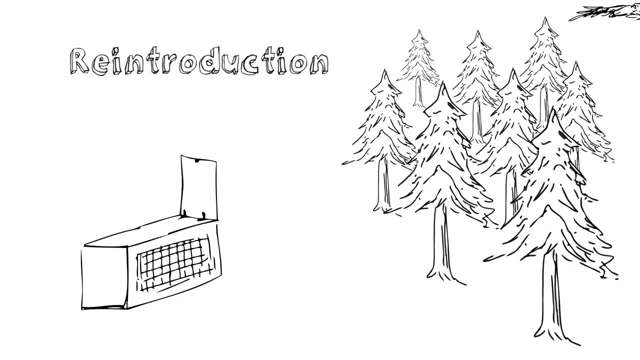 aimed at trying to maintain populations of species that may or may not still exist in the wild. Some SSPs are specifically aimed at reintroducing these species back to the wild. I should say a few brief words on the concept of reintroduction. It's a bit like any high-risk. 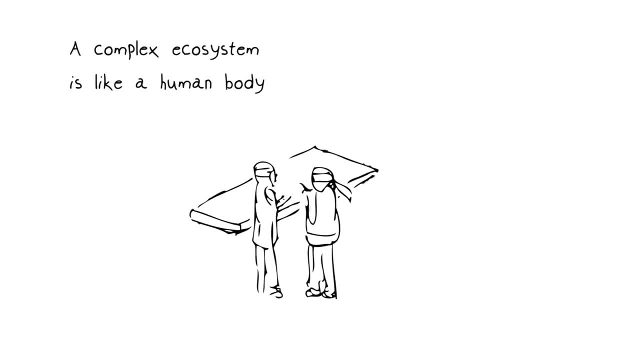 surgery. A complex ecosystem can be compared to your own body. With surgery, it's hard to know if it's going to be successful or maybe introduce more problems down the road, and it's always bloody expensive. Same with programs that reintroduce species that are. 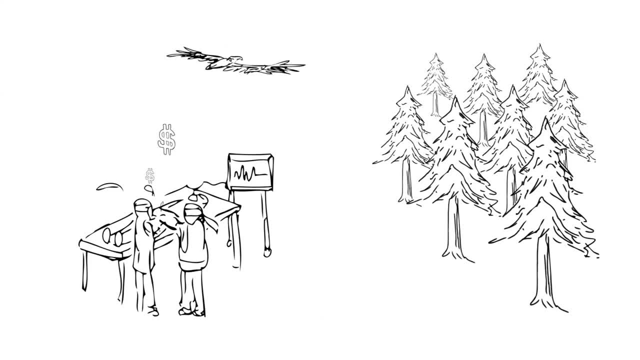 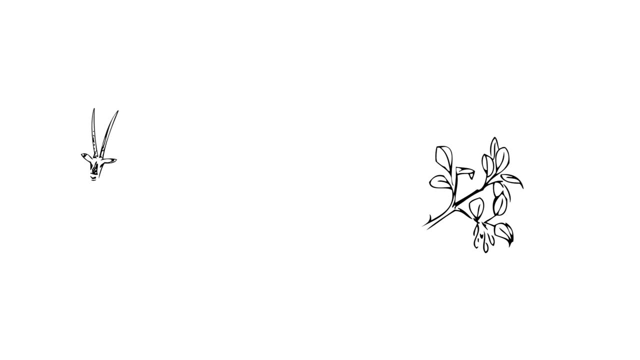 wild in the wild. They may be risky and expensive too, But also like surgery. in some cases, reintroduction can be really effective as a last resort to save lives. It's slowly working – for things like some species of rare plants, the oryx and the whooping cranes. 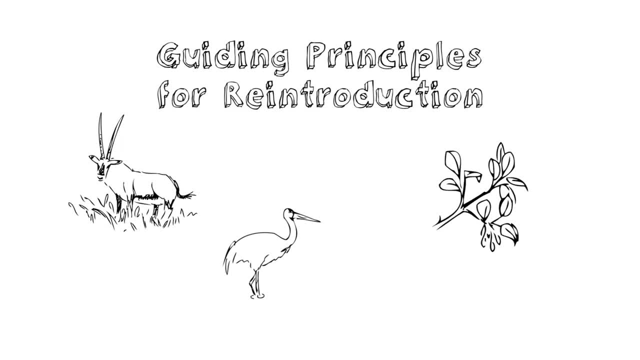 There are guiding principles for reintroductions. There has to be adequate, appropriate, intact habitat in which to actually reintroduce the species. It's important to know which species you're reintroducing. It's important to know if they pose a risk or a risk to the. 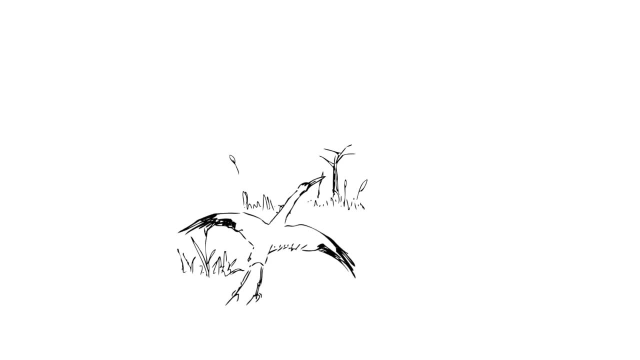 species you're reintroducing, It's important to know if they pose a risk or a risk to the species you're reintroducing. It's important to know if they pose a risk or a risk to the reintroduce the species. So here we get this overlapping effort, not just to save an individual. 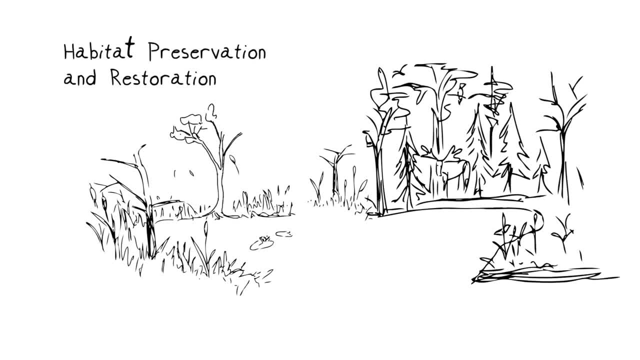 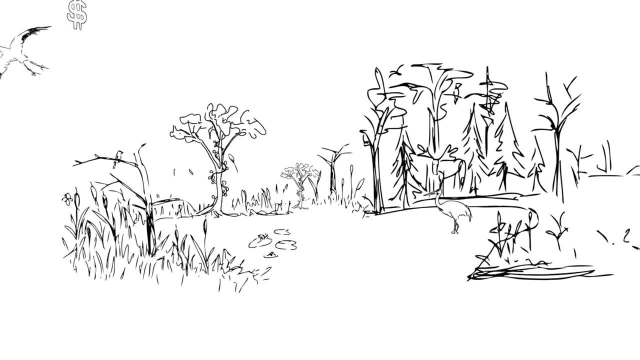 species. but to start talking about habitat preservation and restoration, It's not much good to set your hooping cranes free in the wild if there's not enough wetland for them to dance around in, to mate, breed and get food for their young to let them do their thing. I would insist. 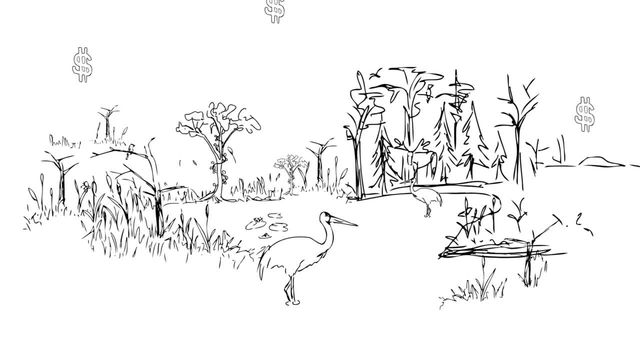 that the expense that we put into these efforts are worthwhile at every step of the way, because of so much more than just counting up the individuals that you can save. The hooping crane is a magnificent animal. It symbolizes something special about unique environments and wild places. 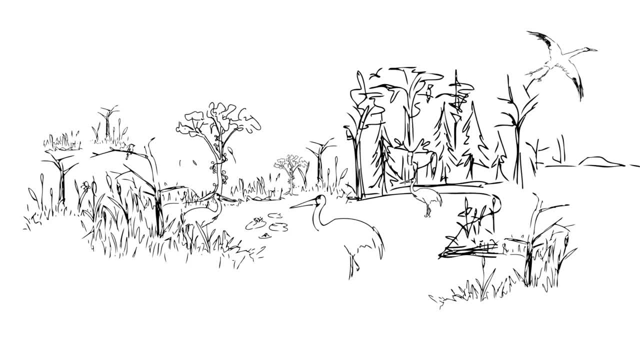 that, in general, people really want to hold on to People like magnificent animals. These cranes focus attention on organisms that symbolize the importance of trying to save not just individuals but also animals, And that's what we're going to talk about today. 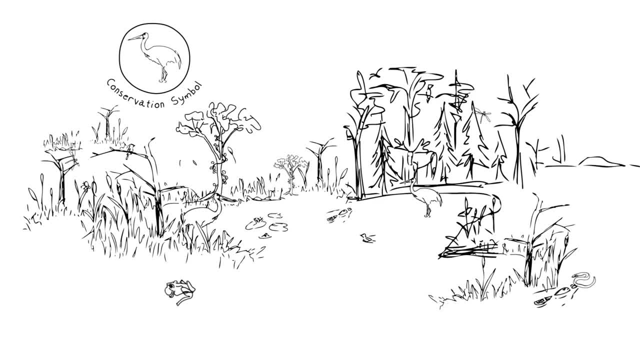 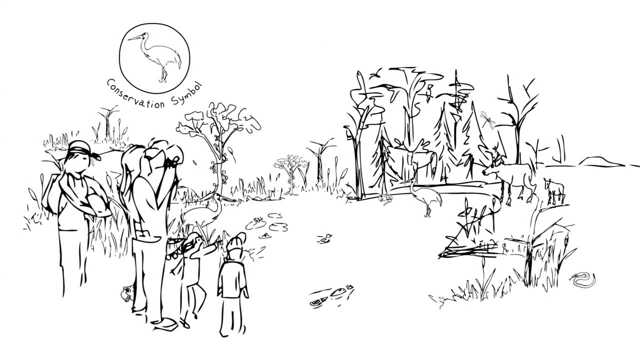 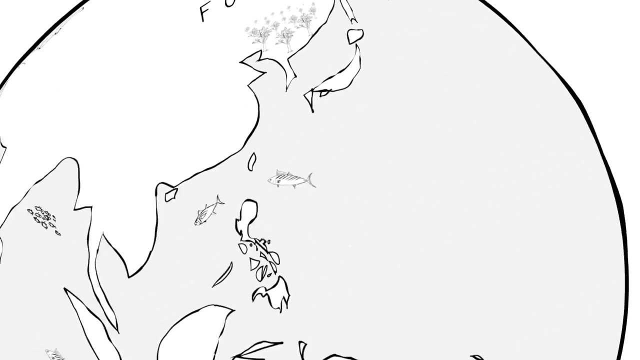 of certain species, but entire places where these species can continue to exist, And the side benefits of this kind of conservation. this technique of reintroduction includes public awareness, a teaching opportunity that focuses even more awareness on the overall problems of biodiversity loss. Let's explore more about what it means to conserve places in nature. 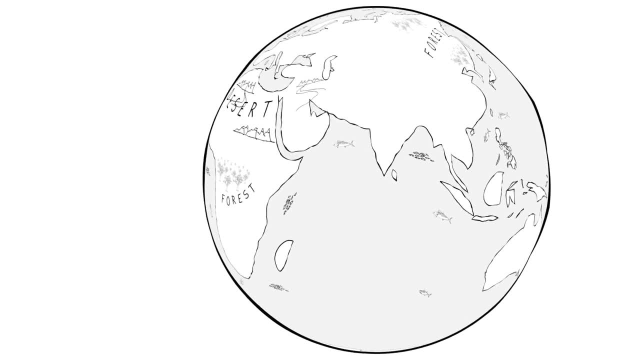 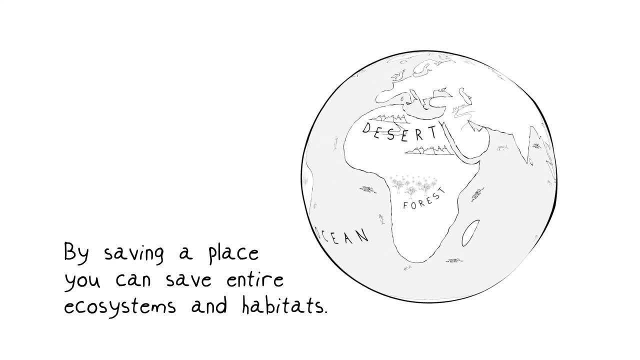 Arguably this is the most powerful way to preserve nature And it's the most powerful way to protect biodiversity, because by saving a place, you will likely be saving entire ecosystems. You're certainly saving habitats, And this approach presents an opportunity to protect. 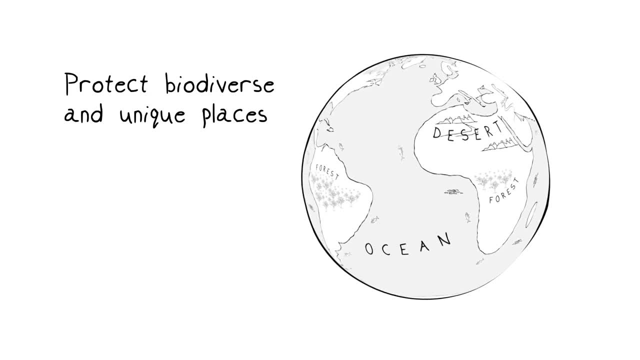 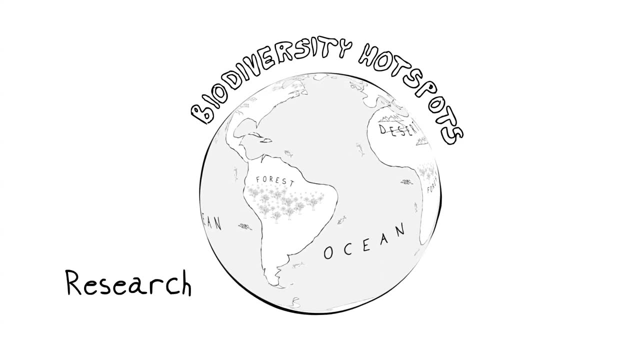 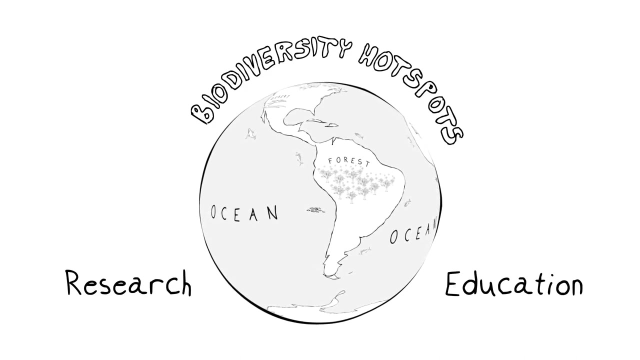 the most highly biodiverse or unique places on earth through the enactment of public policy, Places like biodiversity hotspots. Again, this brings research and education together to help promote and expand the idea of saving an entire place. Now some places have been protected simply by the remoteness. Think of Antarctica, for example. 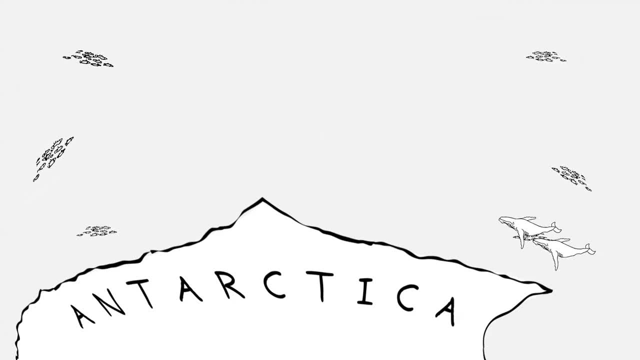 In spite of seeming to be harsh and lifeless, it's a fragile place, full of life, and it's constantly under pressure from some kind of resource extraction, like fishing. Luckily, so far, Antarctic biodiversity has been able to avoid most of the damage caused by human activity, But really only because of its distance from most human activities. 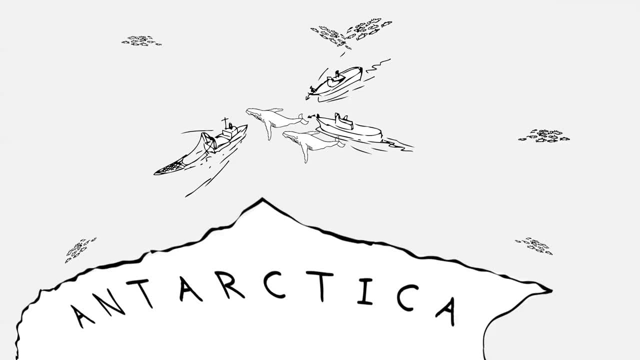 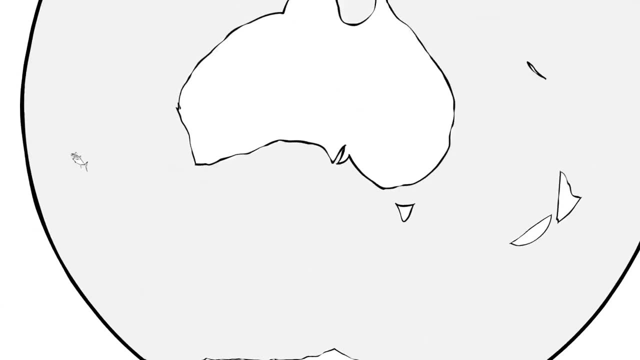 a more difficult place to get to and to make money in, But that will change as technology improves, so that the passive protection of remoteness will likely soon go away. Of course, other places that are more threatened by human encroachment have been singled out for. 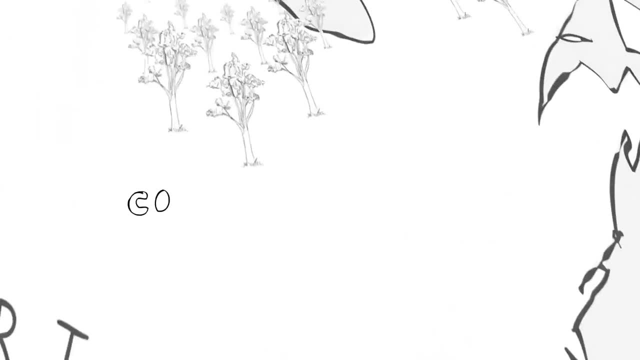 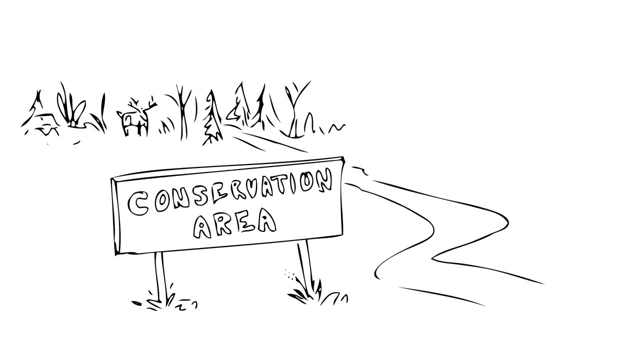 special status as protected parks. I remember in my youth we even had places called conservation areas in southern Ontario where I grew up. Certainly as a kid I loved being able to walk through these conservation areas and seeing things that I wasn't going to see in. 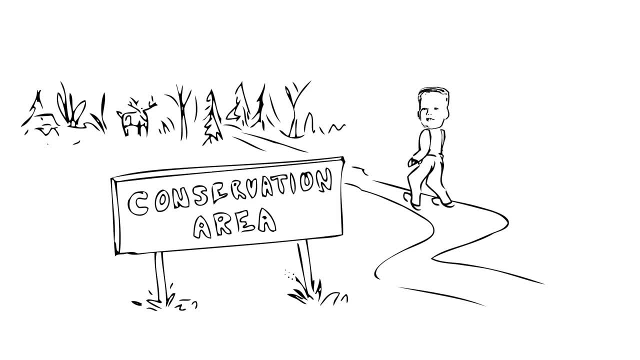 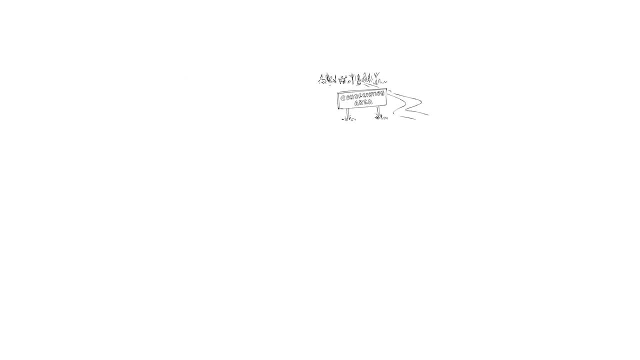 any urban environment that surrounded them. They had a big influence on my early ideas and hopes to study and protect these special places. Everybody knows about the United States National Park System, which has been called America's best idea. It could be argued that without the protected parks and regions that have been established around the world, 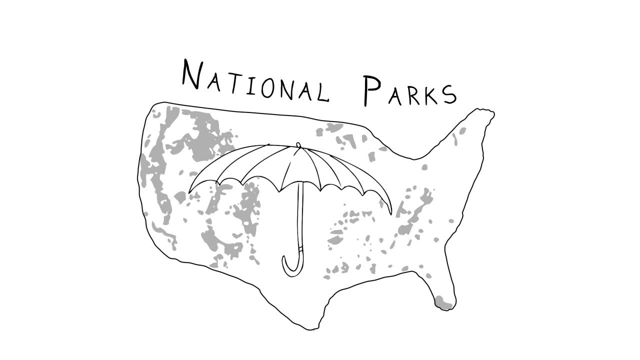 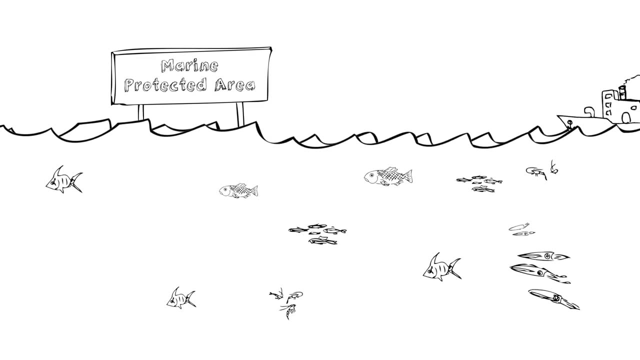 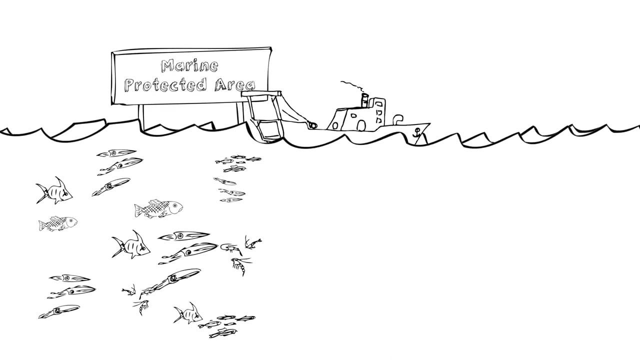 biodiversity would have taken an even bigger hit than it has so far In the sea. marine protected areas are underwater conservation parks. These places are havens for organisms like fish that would otherwise be subjected to over-harvesting that would reduce diversity and cause negative changes in their ecosystems. Marine protected areas can allow. 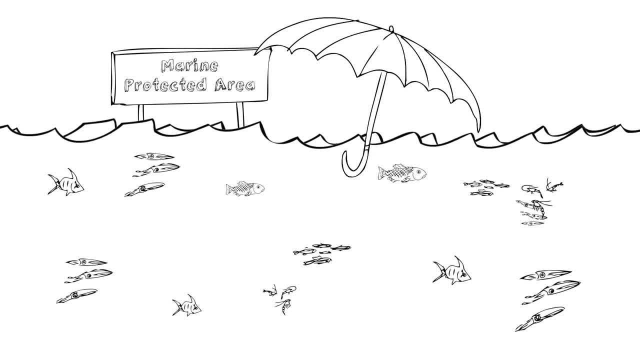 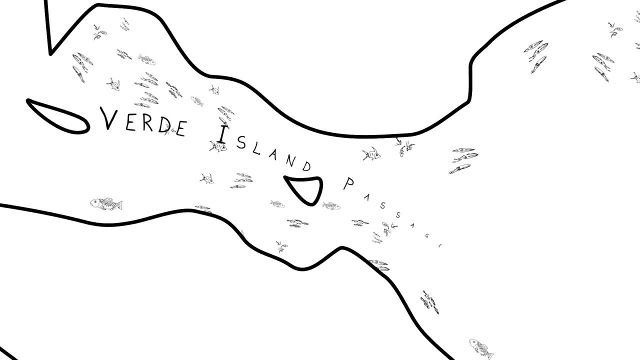 populations to recover, serving as reservoirs to repopulate surrounding areas. A good example of this is in the Philippines, where a body of water called marine protected areas is being used as a source of water for marine conservation. In the Philippines, a body of water called 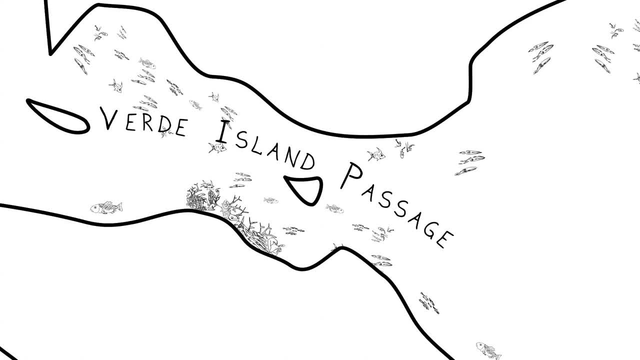 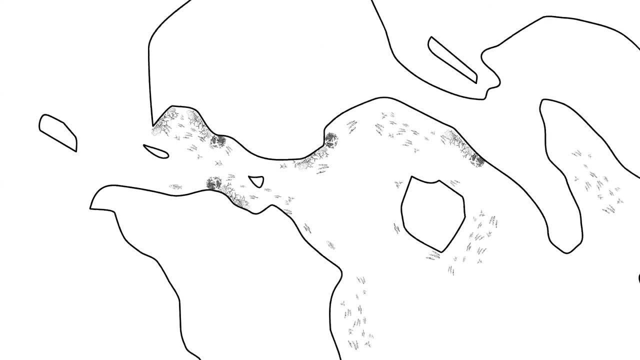 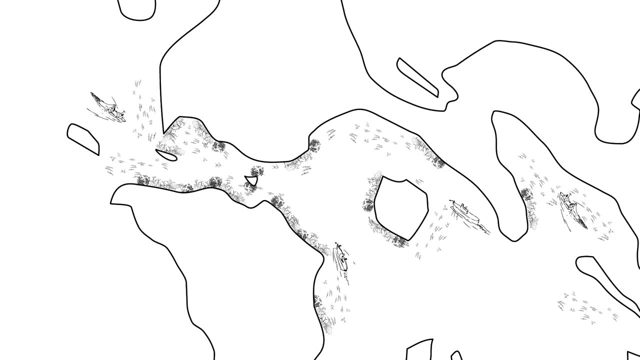 the Verde Island Passage already has patches of coral reef ecosystems that are marine protected areas, But imagine if the entire passage could become a gigantic area where the recovery and reservoir functions can happen. With regulation, total exploitation of this special part of the coral triangle could be prevented, allowing the passage to act as a kind of pump for corals and 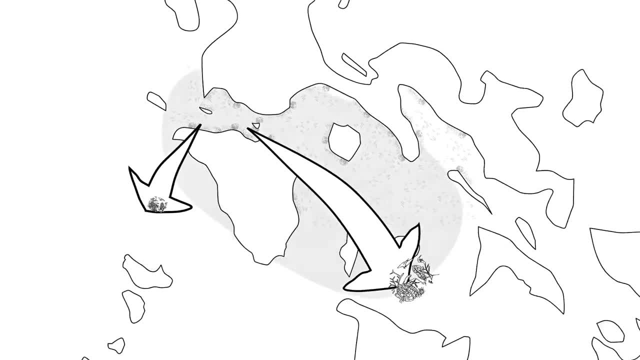 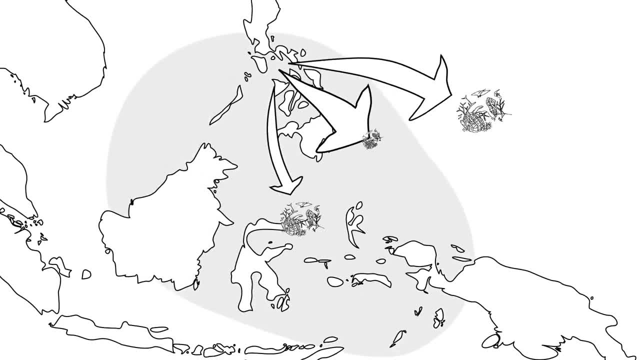 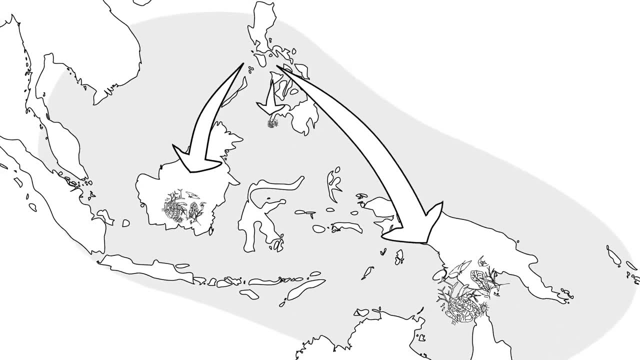 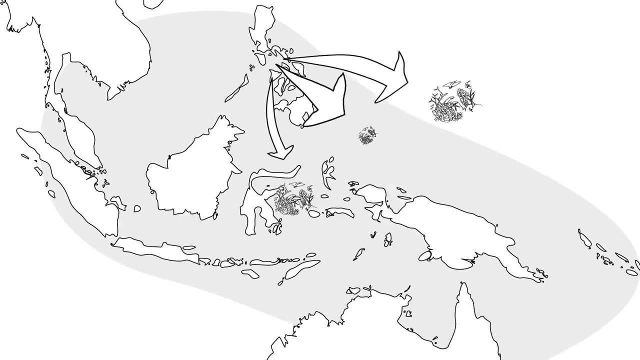 impacted areas in surrounding waters. The Verde Island Passage has shown resilience to coral diseases and bleaching, and surrounding areas suffering from environmental degradation would recover more quickly because you've got this unsurpassed biodiversity reservoir in the Verde Island Passage as a neighbor, A neighbor with that all-important healthy ecosystem function. 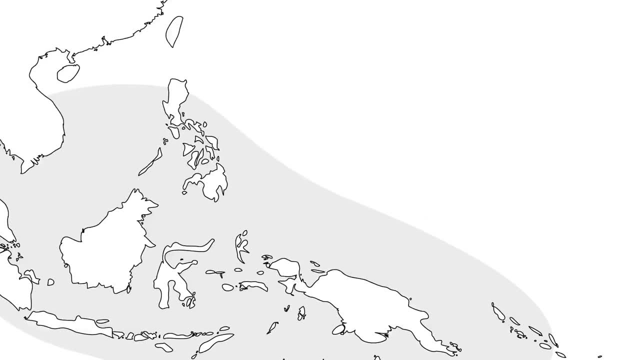 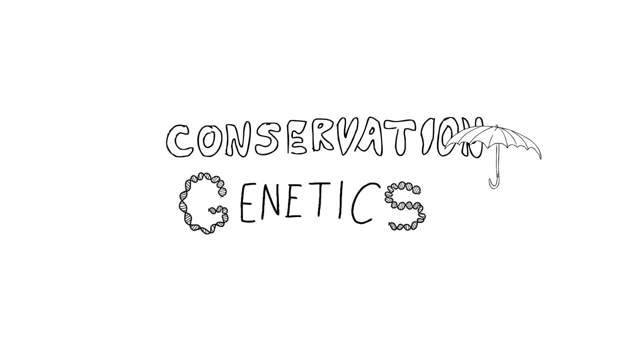 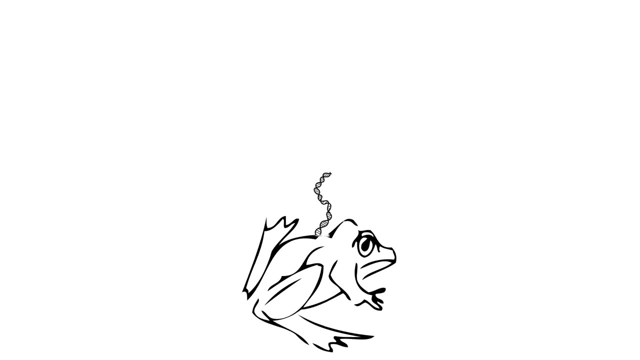 that makes for strong ecosystem services. Lastly, I want to mention and emerging field called conservation genetics. that ties into protection not just of species but of several different levels of biodiversity, from the genetic traits that vary among individual members of populations all the way to the various populations that make up a species, And of course, this includes the.